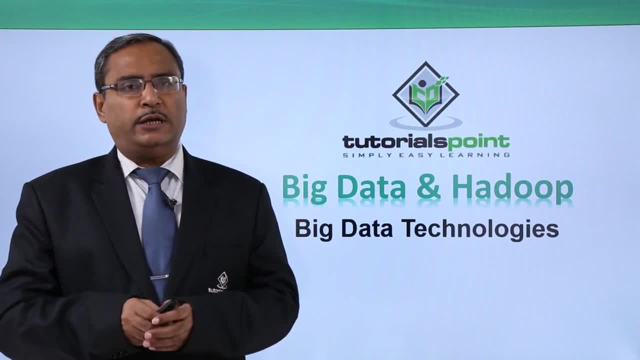 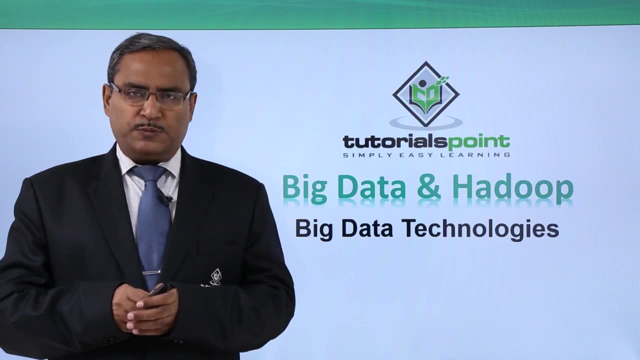 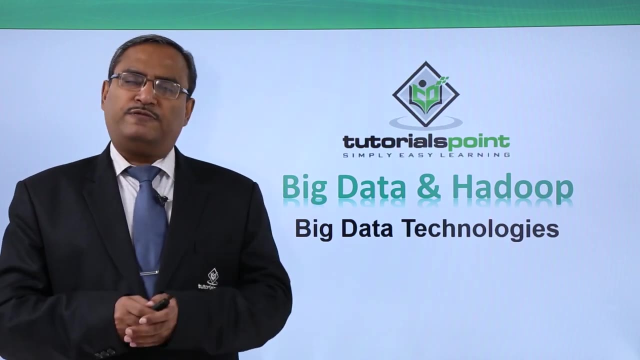 do the strong conclusion and accurate conclusion and prediction, and that will become more effective for the risk reduction. Big data technologies provide mainly two services, that is, the operational big data and analytical big data. So let us go for further discussion on this topic. 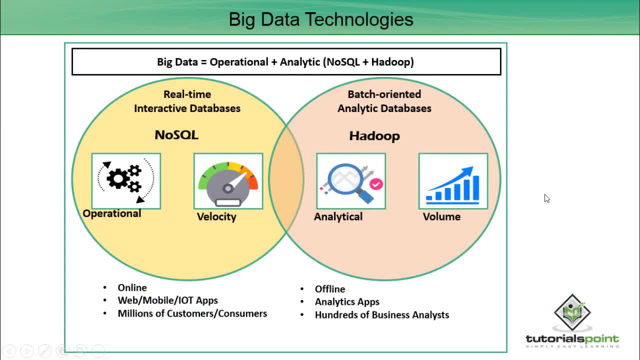 into more details. In this session we are discussing big data technologies. So at first we shall discuss what is big data technologies, And we know that big data technologies can be divided into two categories. One is the operational big data and another one is the analytical big 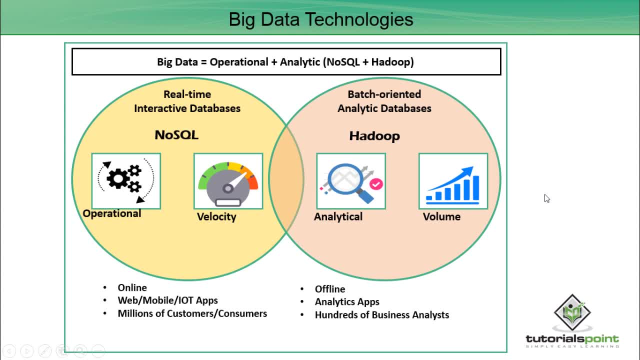 data. So we are going to discuss what is big data technologies, And we know that big data is nothing but comprising of this operational plus analytic, which is consisting of NoSQL plus Hadoop. So what is big data technology? So big data technologies are important in providing more. 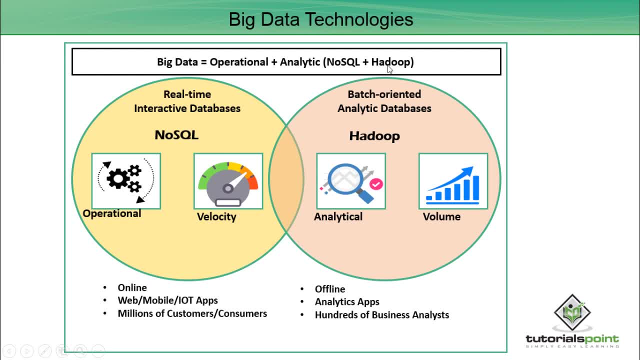 accurate analysis which may lead to more concrete decision making, resulting in greater operational efficiencies. Obviously, we shall go for cost reductions and reduced risk for our business Because, whatever the predictions we are going to make, whatever the operational efficiencies we are expecting and cost reductions we are expecting in the decision making resulting, 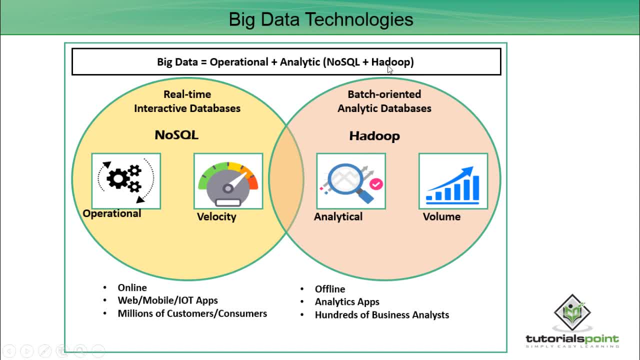 for the better implementation. everything can be obtained in our big data technologies. So there are various technologies in the market from different vendors, including our Amazon. we are having IBM, Microsoft, etc. to handle big data And basically there are two classes to handle. 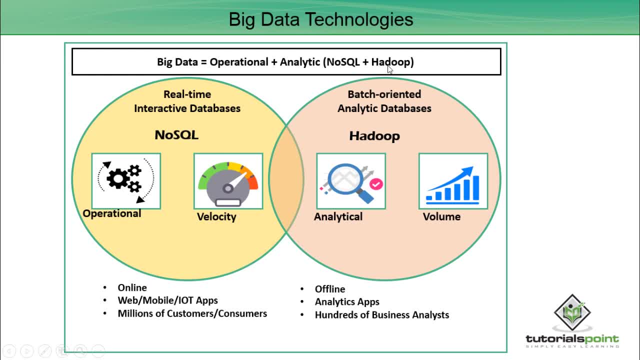 big data. So what are the two classes? So, as we have explained, as we have discussed, that is the operational big data and analytical big data. So at first, we are going for this operational big data which works on real-time interactive databases. NoSQL will be there And we will be. 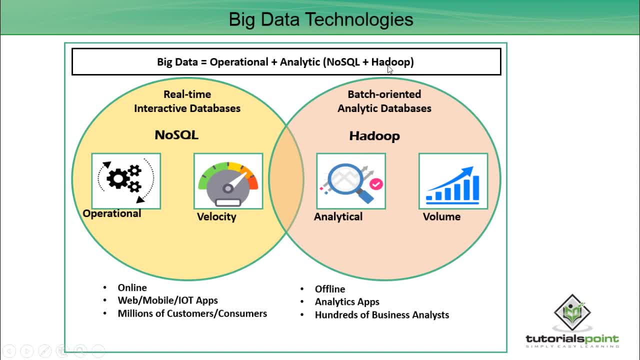 having the huge velocity. that means huge data will be produced. The rate of production of the data will be too huge. So we are going to discuss what is big data technologies And we are going to be working online for the web, mobile and IoT applications And millions of customers and 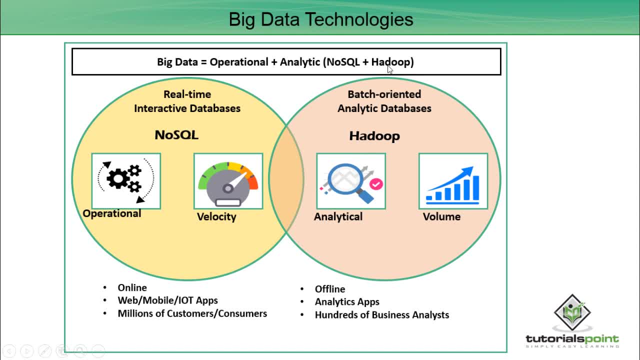 consumers will be related with this operational big data. So this technology is actually the NoSQL database, like our MongoDB, that provides operational compatibilities for the real-time applications, And NoSQL big data systems are designed to take the advantage of new cloud. 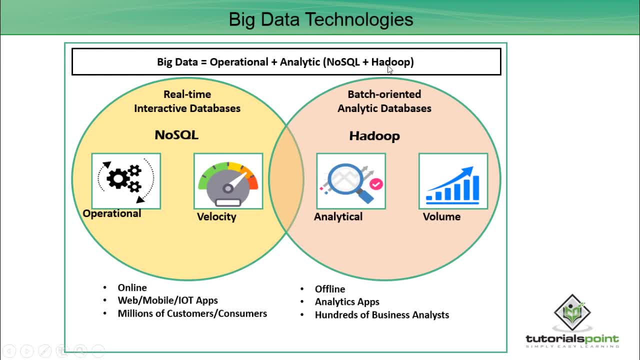 computing architectures that have emerged over the past decade, So we are going to talk about another potential use case of Big Data. It is technology that can not only be used for data processing, and hence rein clutching some sort of a data center, but also allow 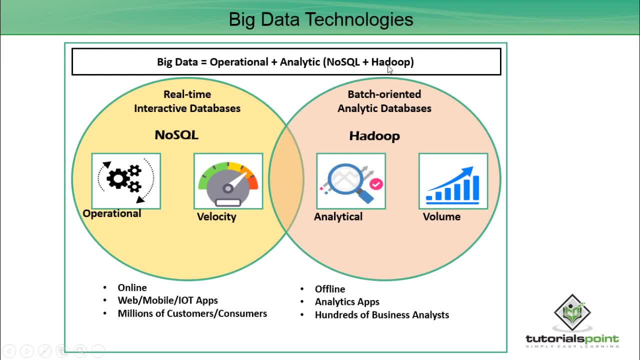 it to be used for all kinds of operation or images which can be run in a routine manner. Tell me about that. Come on, I'm going to tell. this is a really fun topic, really, because I've been reading on a lot of websites about. 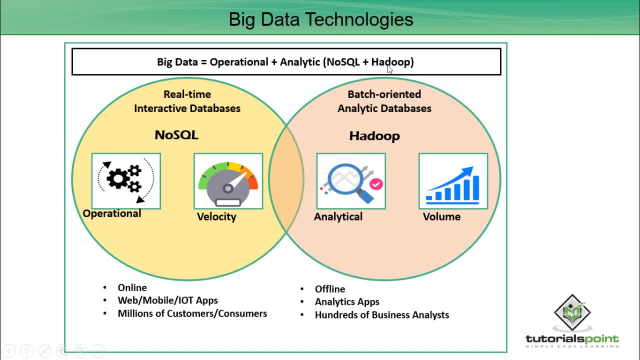 Creative Cloud. So it's such an interesting topic because not only is it about a technology, about a data set, about how you treat a business, It's about all these data centers around the Or we can provide some insights of the pattern in our data without having any additional expenses, without having any additional infrastructure and data scientists. 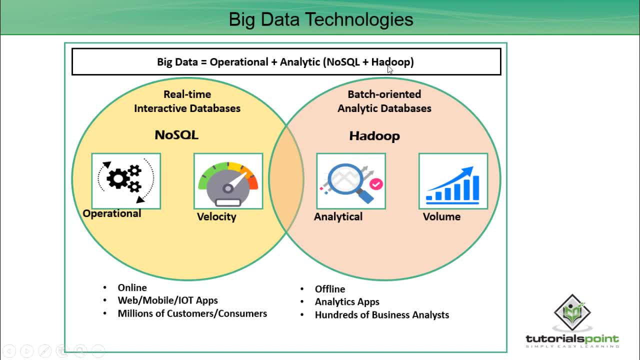 Now, what is the analytical big data? So analytical big data is actually the batch oriented analytic databases. We're going to have our huge volume of data to be handled offline. Analytical applications will be there and hundreds of business analysts will be working on this. this about analytical big data. 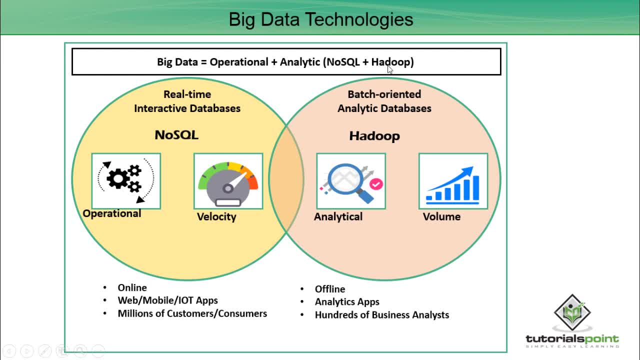 So this includes systems like our massively parallel processing, So remember this term very carefully. There is a massively parallel processing- In abbreviated form we usually call it as MPP- massively parallel processing, database systems and MapReduce that provide analytical capabilities for retrospective and complex analysis that may touch most or all of our data. 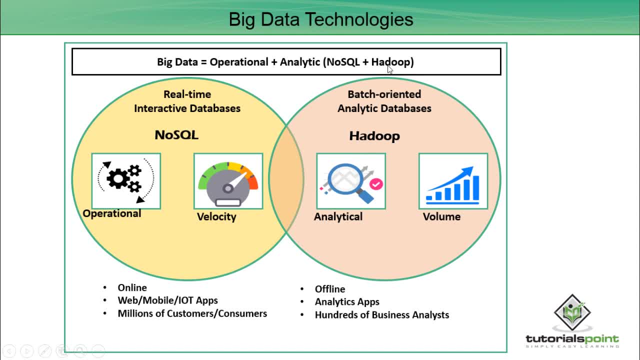 And the MapReduce provides a new method for analyzing data that is complementary to the capabilities provided by SQL. SQL was having some limitations and this MapReduce? It provides a new method for analyzing data and obviously that is complementary to the capabilities provided by SQL, and its system, based on MapReduce, can be scaled up from, say, single servers to hundreds, thousands of high and low end machines.